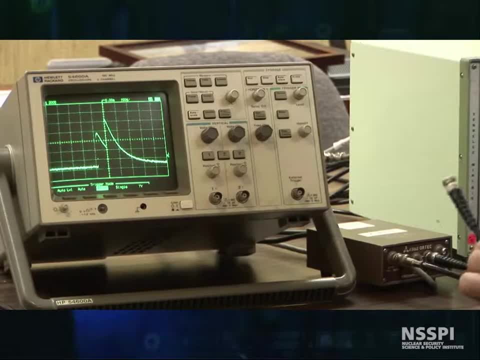 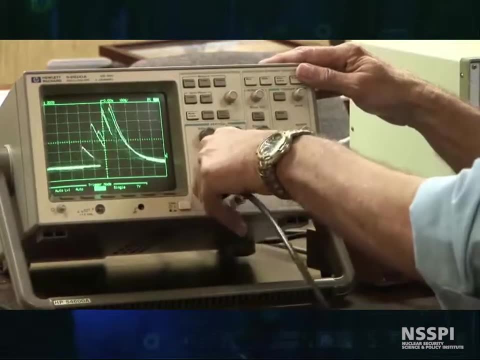 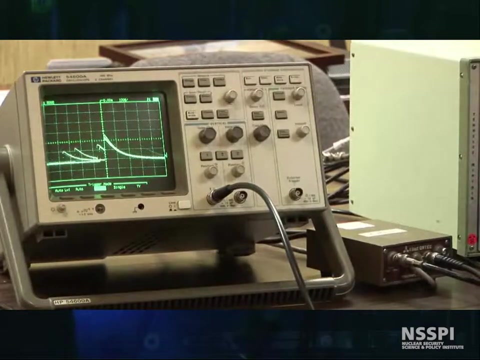 Okay, we've hooked the detector up to a source. It's coming to the preamp And here's what the signal looks like coming out of the preamp. Wow, we've got good pulses coming from the preamp. We have lots of signals. This is set for 100 microseconds, So it takes a couple hundred microseconds for a pulse from the preamp to decay away. 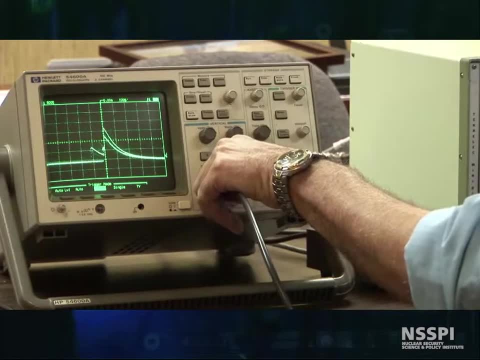 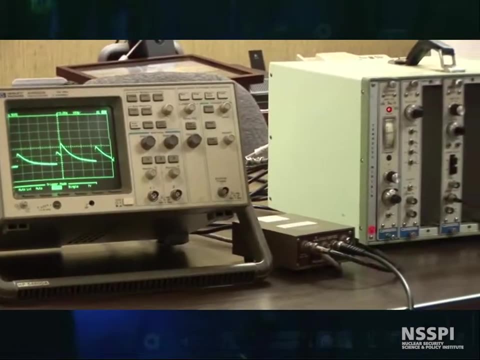 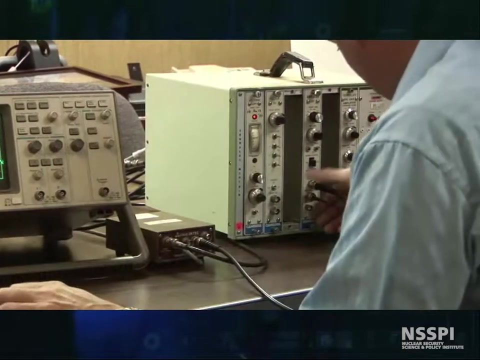 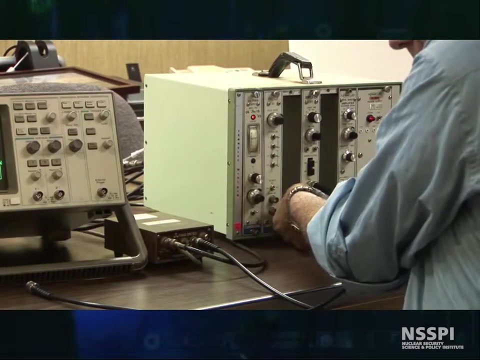 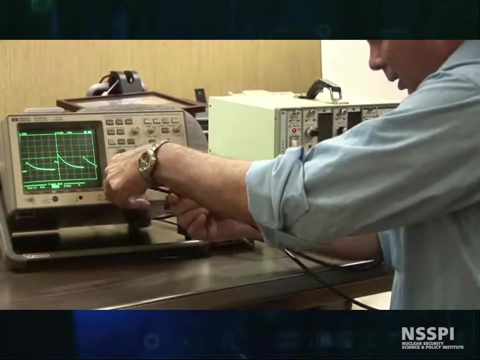 So we're now going to take this and we're going to hook it to the input of our amplifier. All right, If we take the output from the amplifier, we can now look at it with our oscilloscope. Wow, it's bigger, It's faster. 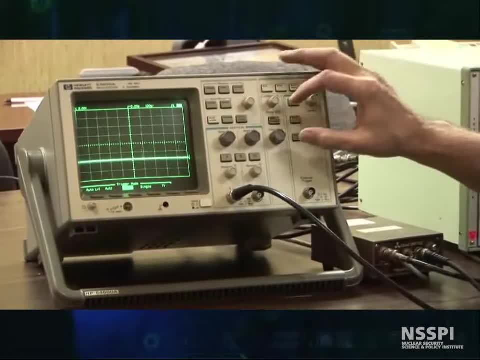 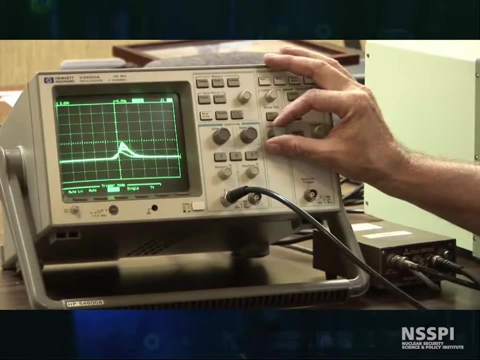 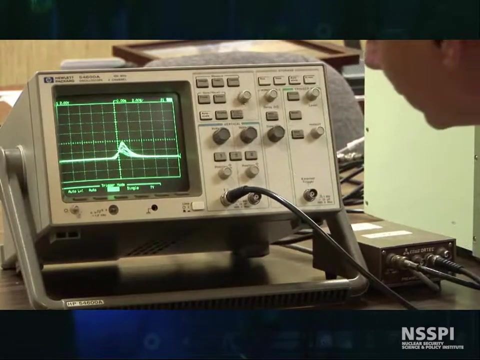 In fact it's so fast. they just are little single ups and down pulses, So let's speed up. Ah, there they are. So this is on a 2-volt scale. I can change this to a 1-volt scale. 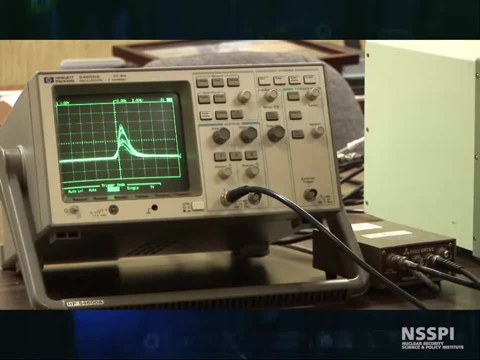 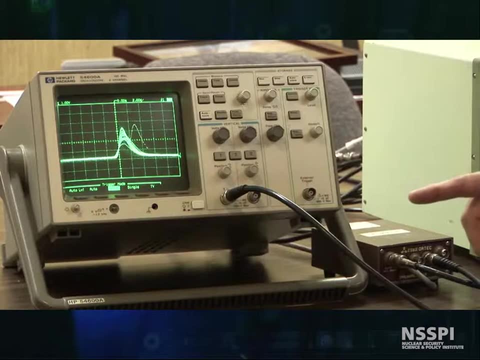 And there we go. That's what the pulses look like coming out of the preamp. All right, And now we're going to take the signal that's coming out of the amplifier. This all looks good to me, so now let's feed that into our multichannel analyzer. 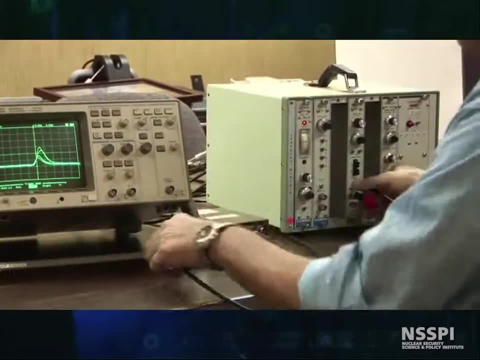 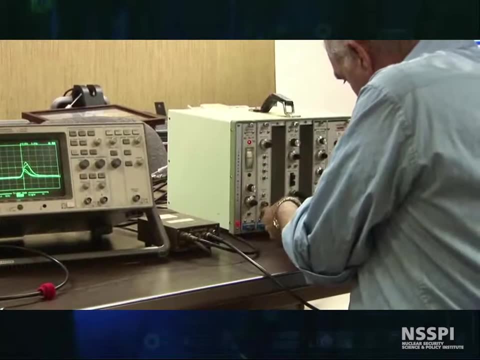 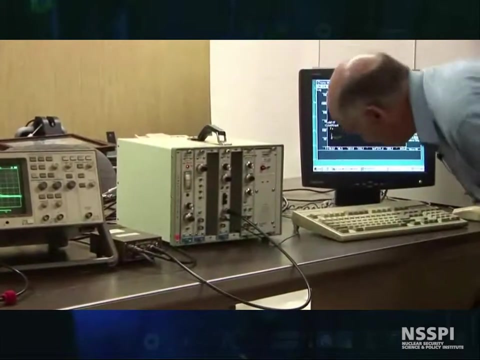 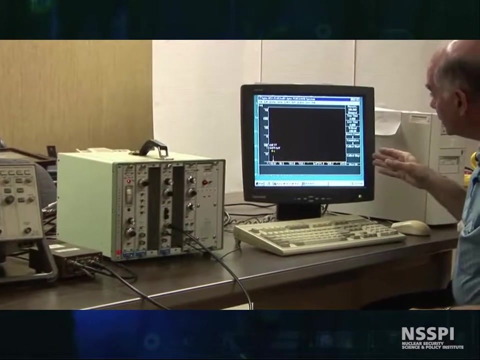 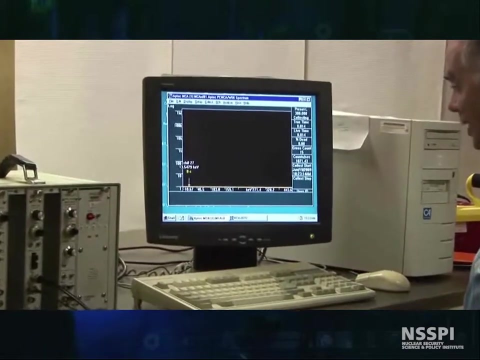 and get a pulse height distribution. Okay, here we are. This is where we're going to build our pulse height distribution, and I can start it. It scans for about a second and then it will begin to display. Oh, here it comes, and this looks pretty good.